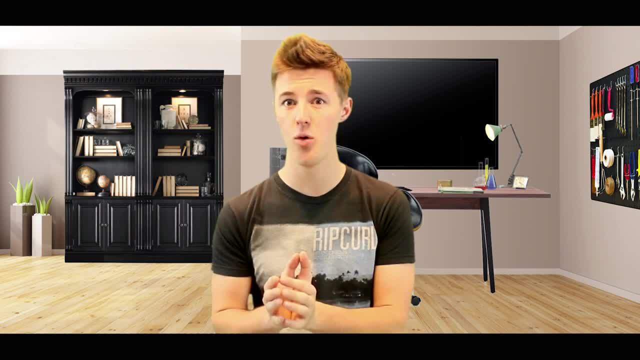 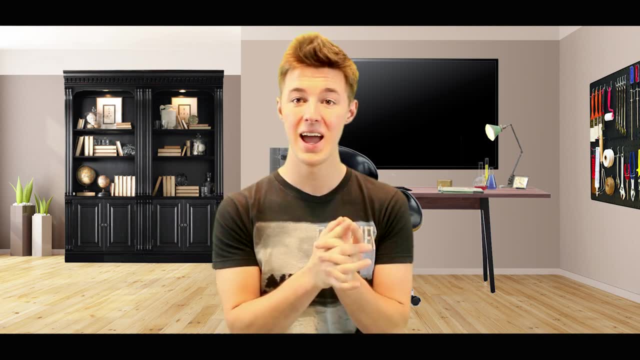 kind of going along that same route. what are some chemicals at home that you should absolutely never mix under any circumstances, And the very very first of those is bleach and vinegar. Now, when you combine bleach and vinegar, they make an actually pretty good. 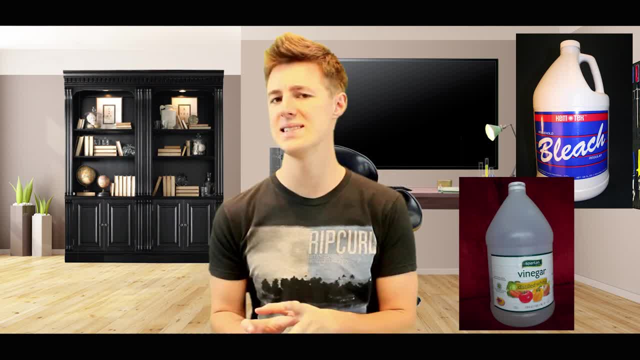 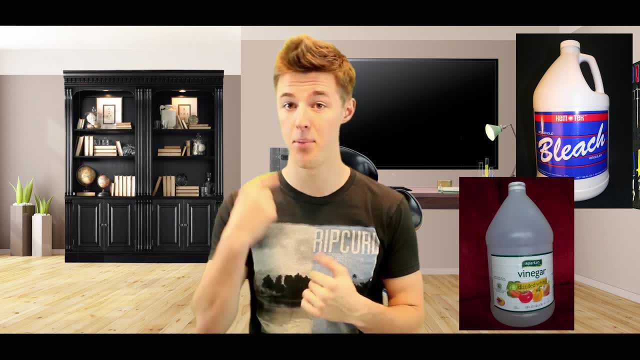 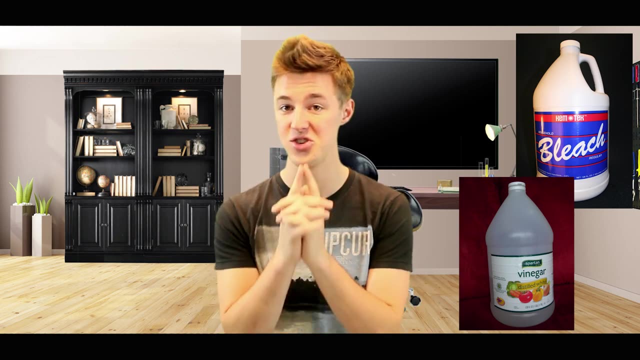 cleaning substance, But when you add any sort of weak acid to bleach, it starts giving off chlorine gas, which is so bad that it can start literally chemically burning your lungs and your eyes And do some really, really nasty stuff to your skin. So it's absolutely should not be. 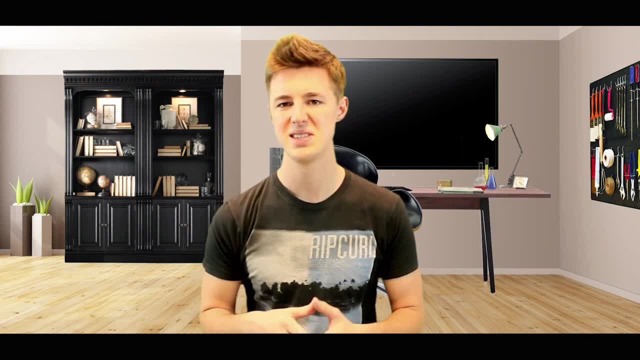 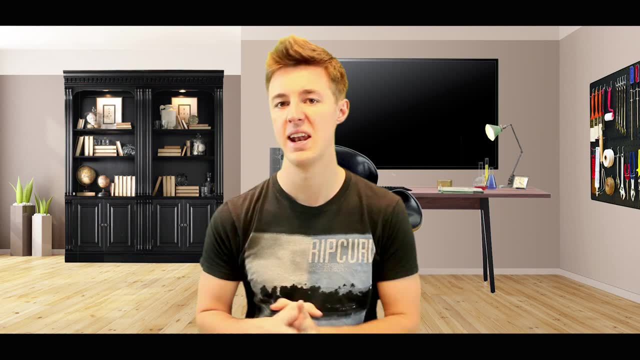 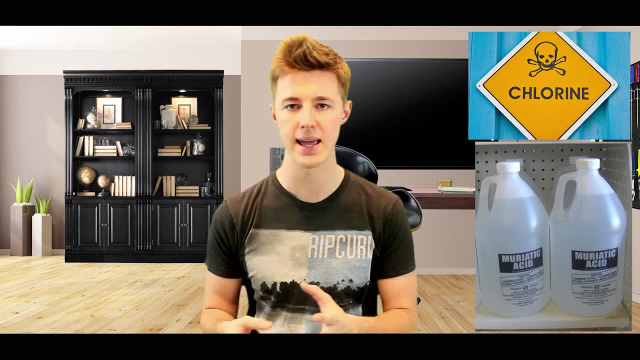 messed with. Chlorine in general is a pretty nasty substance. In fact, you really shouldn't combine anything with chlorine or combine anything that makes chlorine. I clean pools for a long time. And if you combine chlorine tablets with pool acid, which is muriatic acid diluted hydrochloric, 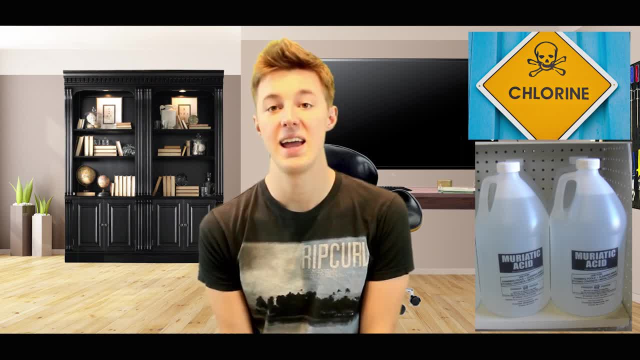 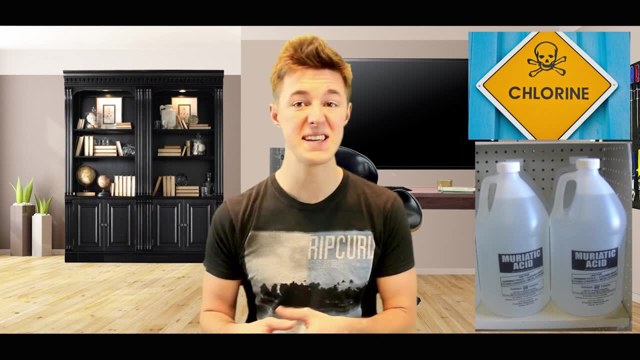 acid. it makes really, really bad things. In fact, it makes really bad things. So I recommend, if you do not have chlorine, you should just mix it with chlorine And, as I said, chlorine is a really, really bad thing If you just mix. 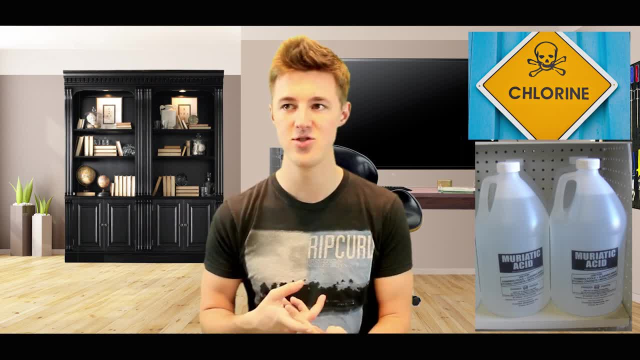 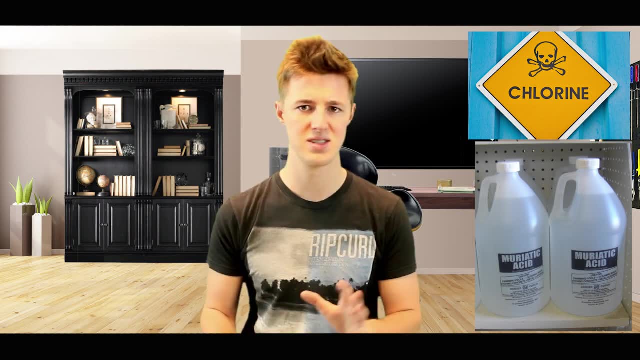 it with chlorine. it can kill your lungs and your eyes, So it's a really, really bad thing. And if you don't have chlorine, you should just mix it with chlorine. And if you don't have a chlorine, you just mix it with chlorine And that's it. 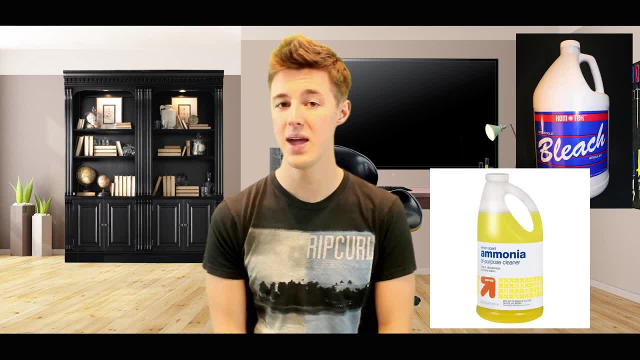 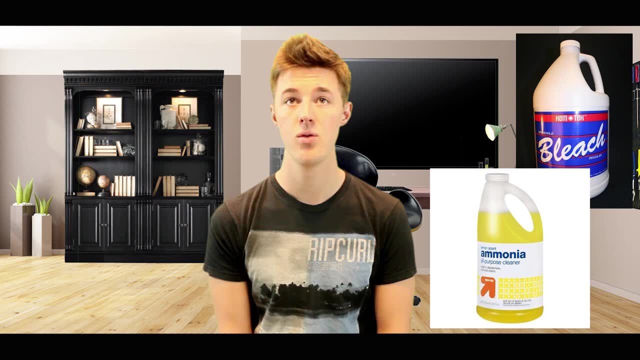 Next up we have a very, very nasty substance. It's called the mustard gas, which is what you used in World War One in trench warfare to kill people. It's what was used in the Holocaust. you quite quickly. It's very, very toxic to your lungs Now. 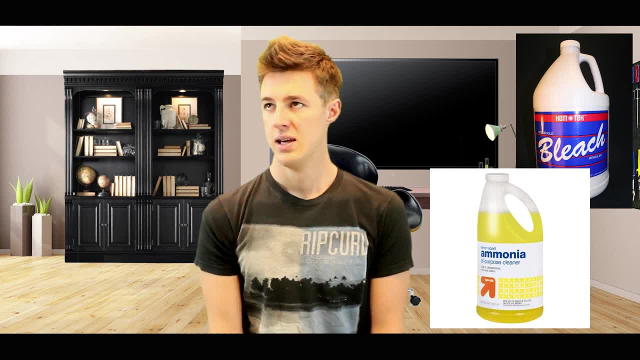 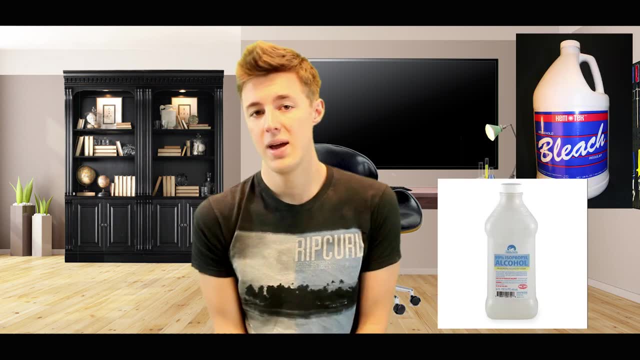 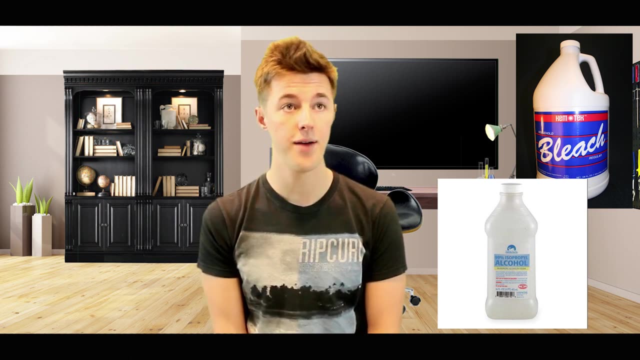 for those of you secret agents out there, you probably already know this, and I hate to give this power to the internet, but simply combining rubbing alcohol and bleach will make chloroform gas which, if you breathe in too much of it, will kill you, like like you know everything else on this list. 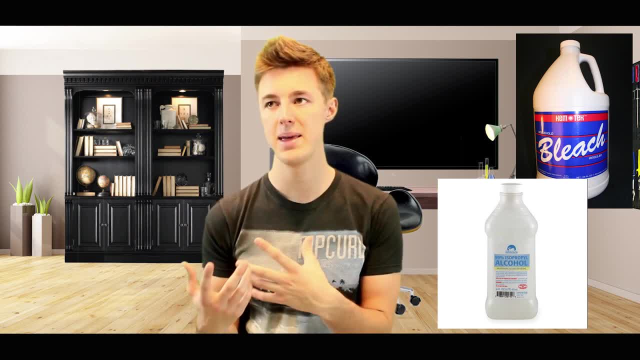 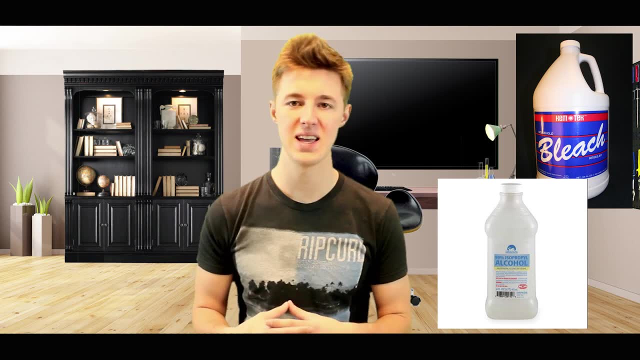 but just breathing in a little bit of it has been used by people for a long time to kind of knock people out in a very, very well, relatively safe manner. Inhaling it decreases your oxygen intake and, as long as you do it for a very, very 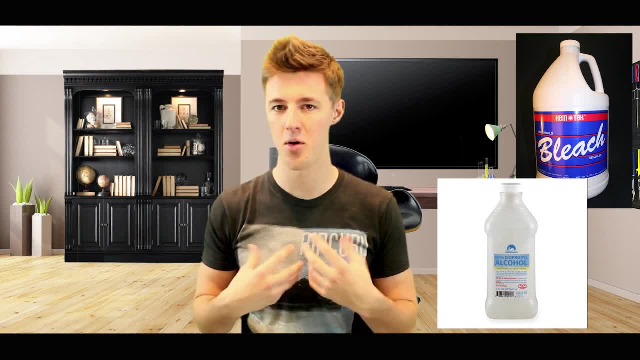 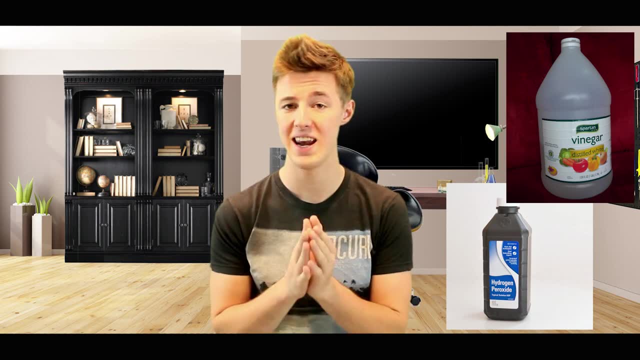 very short amount of time. you're not going to burn anything, but it's still not a great thing to be inhaling and it will kill you if you do it for too long. The next one on our list is hydrogen peroxide in vinegar, which makes parasitic acid. Not much is actually known about parasitic acid. It's not like the other ones where it's probably going to kill you just by breathing it or, you know, create third degree chemical burns on your eyes or lungs, but it will be irritating in. 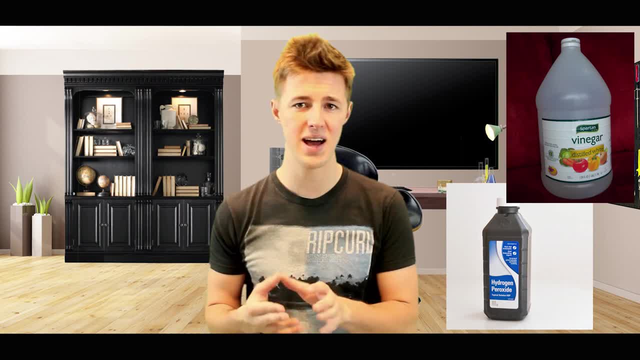 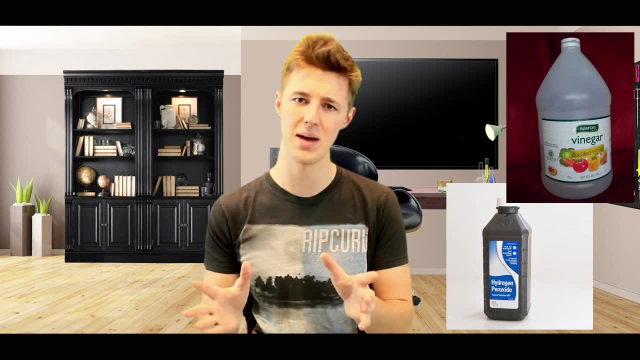 certain concentrations, So it's still probably not a combination you'd like. You can just use the two chemicals at completely different times and you should be fine. Just just don't mix chemicals in general- really, Coming to the sixth item on our list, you literally can get in trouble mixing your 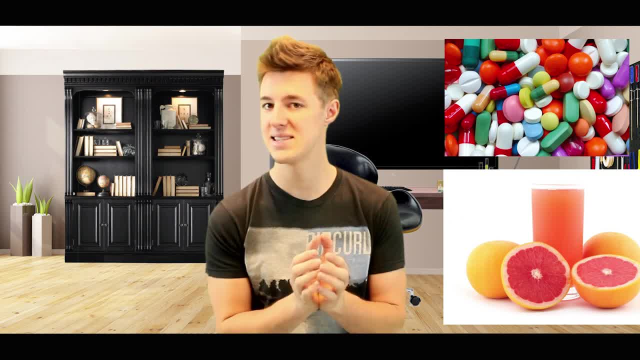 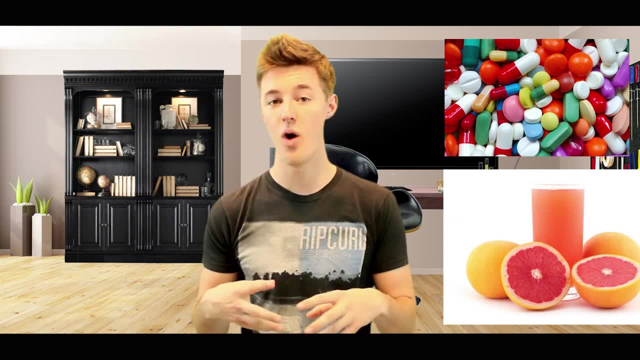 medicine and grapefruit juice. Medicine and grapefruit juice: Okay, it's kind of a big deal because grapefruit juice makes you absorb chemicals faster. So if you have a certain concentration that's supposed to be released in your body at a certain speed and you drink, 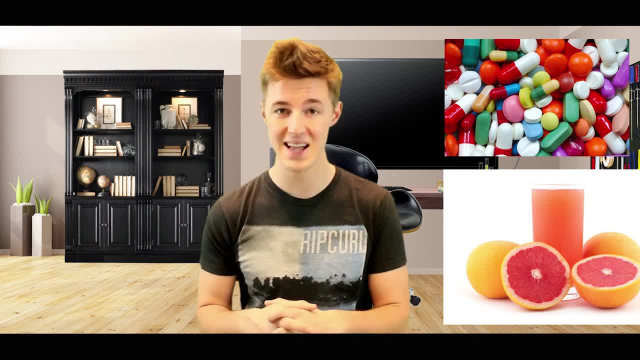 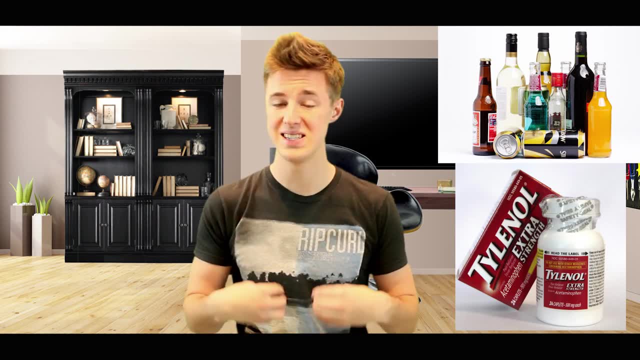 too much grapefruit juice, you could start overdosing and that's not good at all. and the next reaction is acetaminophen- I think I said that correctly- in alcohol, which when you combine the two, it can actually damage your liver to the point where it more than likely will fail, In fact, about. 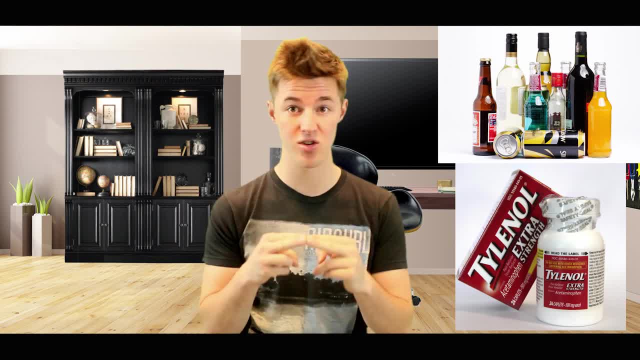 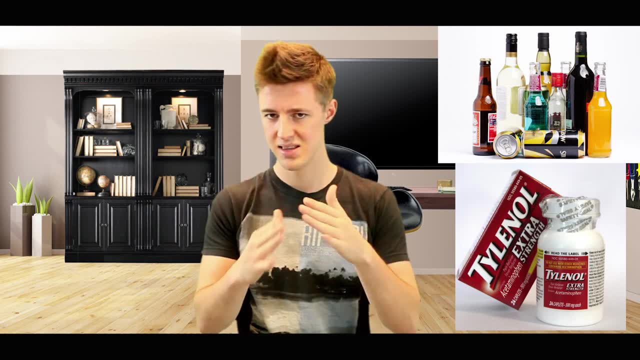 200 deaths a year happen just from this particular combination of chemicals. It's really not something to be messed with. So don't take drugs and drink folks. It's not not a good combination there. And finally, is ibuprofen in? 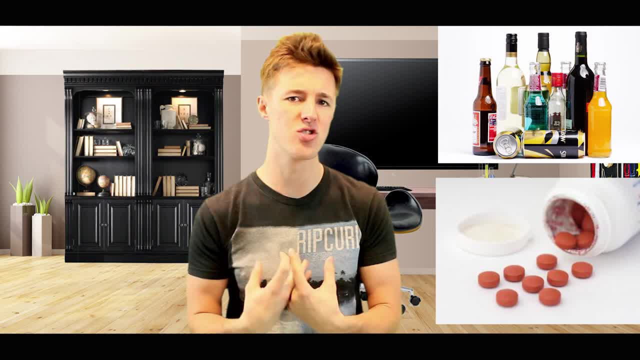 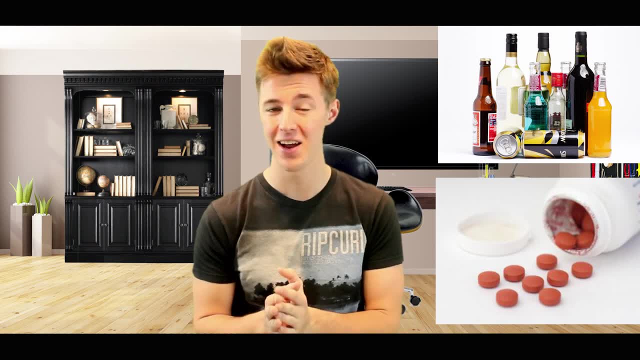 alcohol. The two combined can actually tear up your stomach lining, and if you have a propensity to get stomach ulcers it can be even worse. You can really cause a lot of problems in there. If not, it may not happen, but still not. 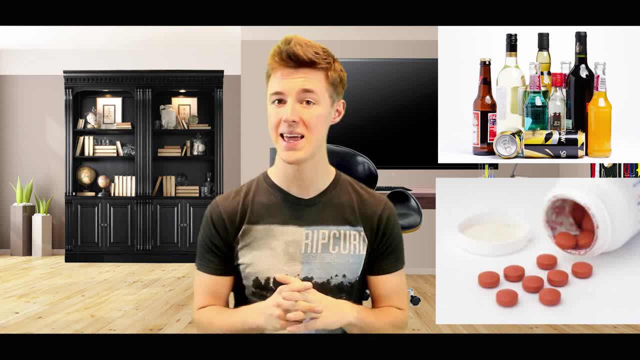 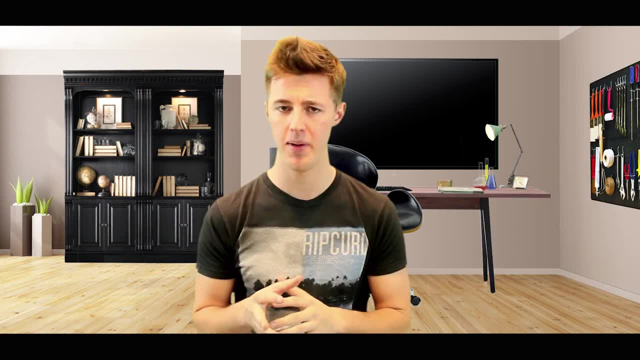 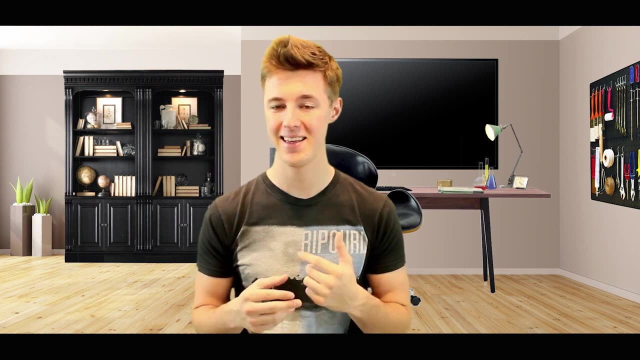 advisable for you to be able to get stomach ulcers If you're going to be doing anything with combining chemicals, in fact, kind of a random chemical connection, it's not on this list and it's not exactly confirmed by any sort of company or, you know, laboratory or university or anything like. that, though it has been confirmed by a junkie website, and something I personally went through a little while ago was: I went to Florida and I was feeling sick and I decided to take a full dosage of NyQuil, which normally I only take a third of a dosage of NyQuil. Anyways, I took NyQuil and the 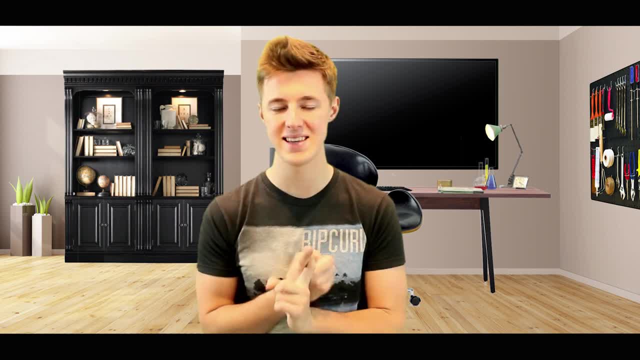 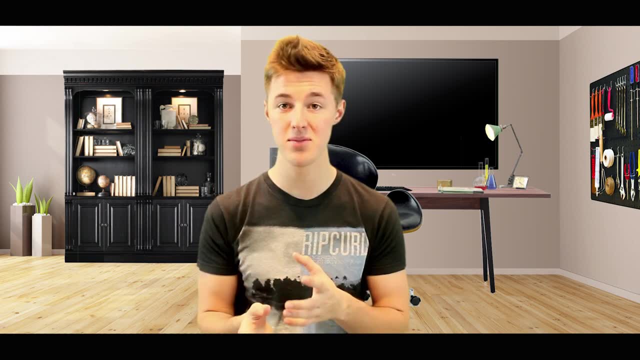 primary ingredient in that is shortened to DXM. I also had a ulcer in my mouth and I was using this stuff called Ambasol. Well, Ambasol has this chemical in it called Benzocaine and apparently, according to junkie websites,